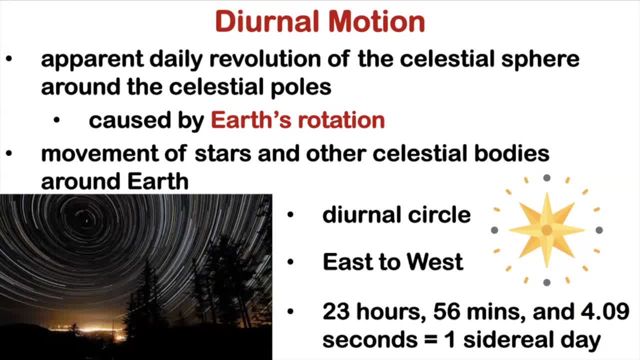 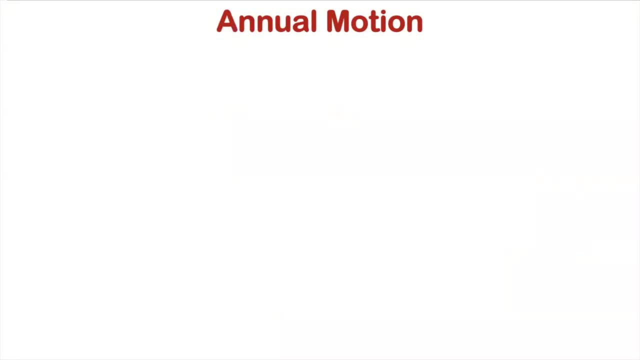 So this is what we call a one side real day. So that's it for diurnal motion. We also have what we call the annual motion. So, based on the word annual, it's by year. Okay, this is the apparent yearly movement of the stars as observed from the earth. This one is caused by the earth's revolution. 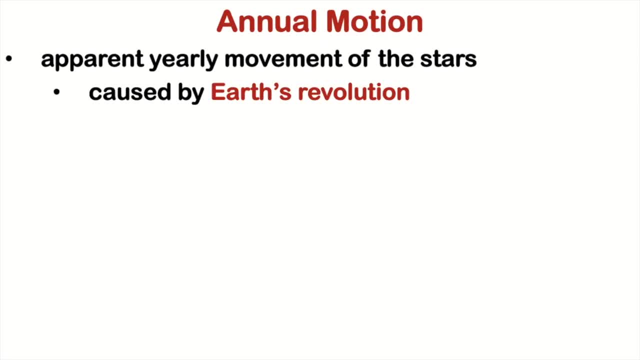 Again diurnal, caused by its rotation. annual, caused by its revolution. So the sun revolves around the celestial sphere with its path being called the ecliptic. As the earth moves around the sun, the apparent position of the sun in the sky changes. This change results in the changes to the 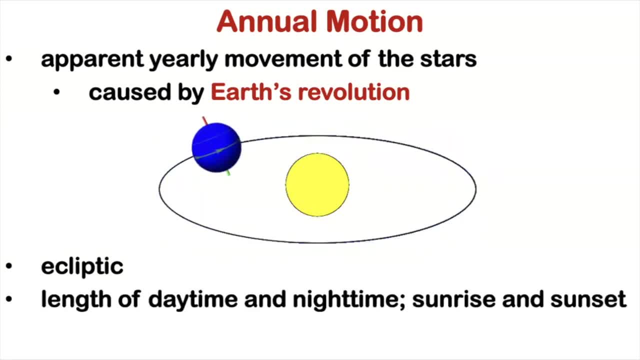 length of daytime and nighttime. This change results in the changes to the length of daytime and nighttime, As well as the changes to the sunrise and sunset points. So these changes are responsible for the different seasons we experience throughout the year. Well, aside from climate change, Lastly, we have the 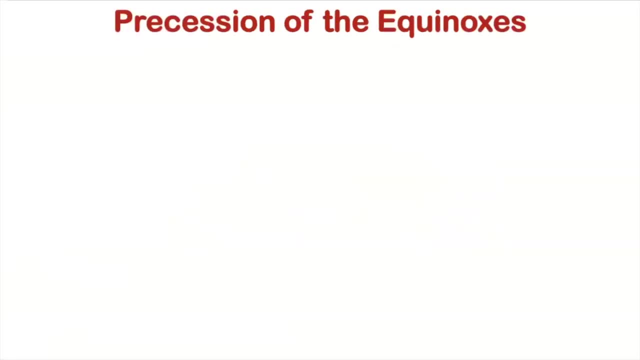 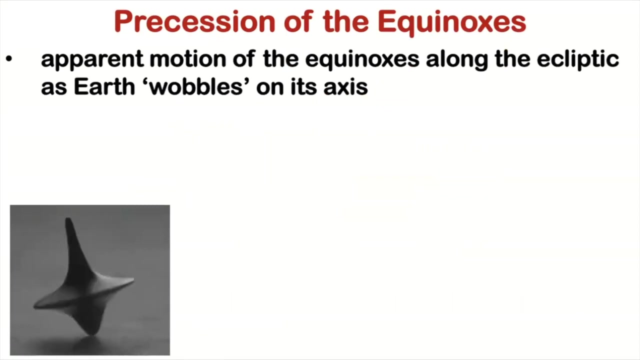 precession of the equinoxes. Okay, to put it simply, it's a slow, gradual wobbling of the earth's rotational axis. Just imagine spinning a top and the top started to wobble. That's kind of what's happening. 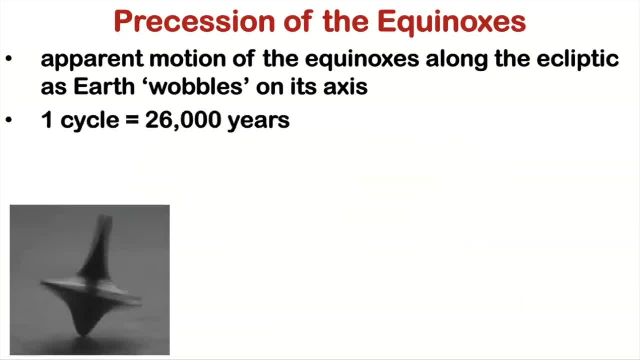 to the earth. So the precession of the equinoxes takes about 26,000 years to complete one full cycle. Now you have to remember that as the earth wobbles, the position of the stars in the sky appears to shift over time. So this means that over the course of several 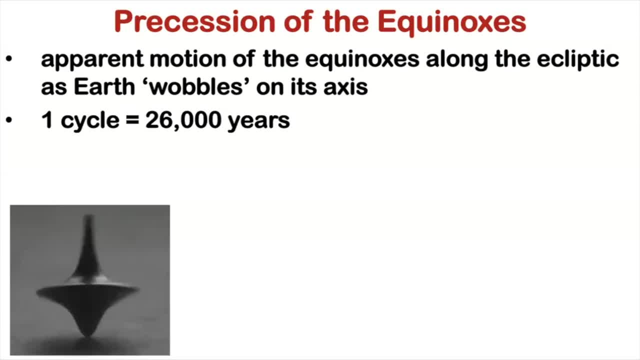 thousand years, the constellations we see in the night sky will appear to move slightly. Okay, for example, let's take the constellation of Libra. Right now it's located in a certain part of the sky, But in a few thousand years,